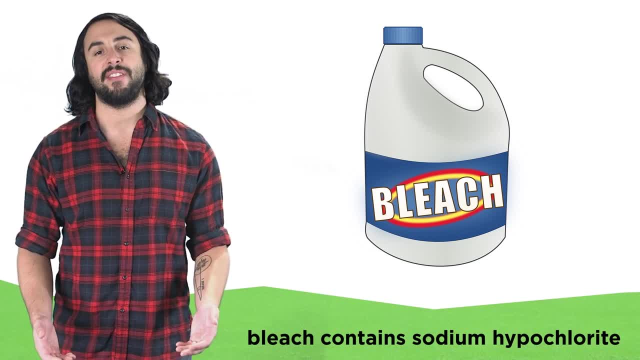 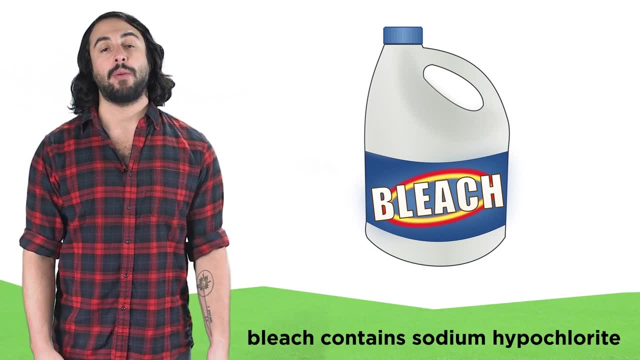 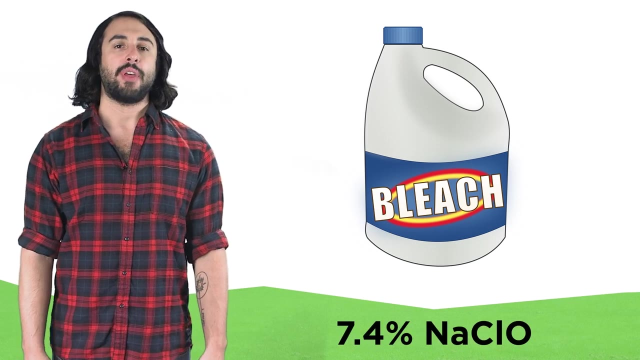 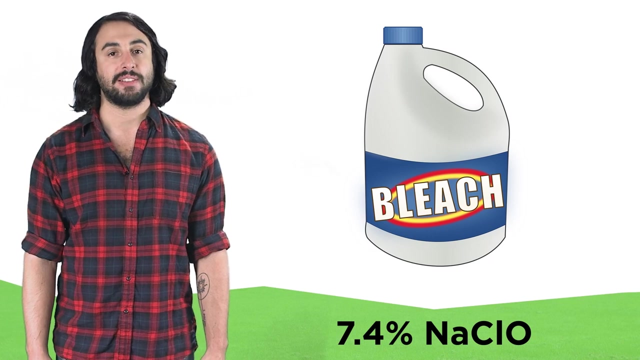 Take, for example, a typical bottle of bleach. The active ingredient in bleach is sodium hypochlorite, and we might commonly see the concentration on the bottle listed as being 7.4%. That means that this is an aqueous solution consisting of 7.4% sodium hypochlorite by 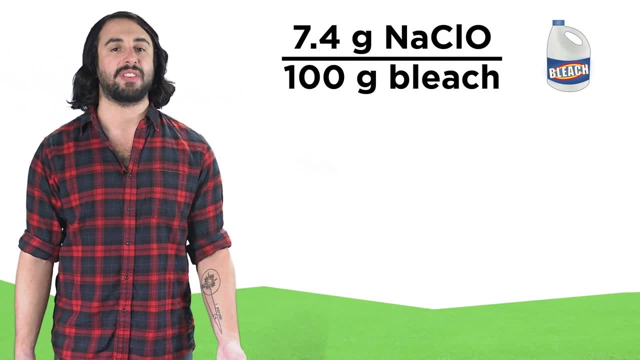 mass. In other words, if there were a total of 100 grams of bleach, 7.4% sodium hypochlorite would be mass. That means that this is an aqueous solution consisting of 7.4% sodium hypochlorite by. 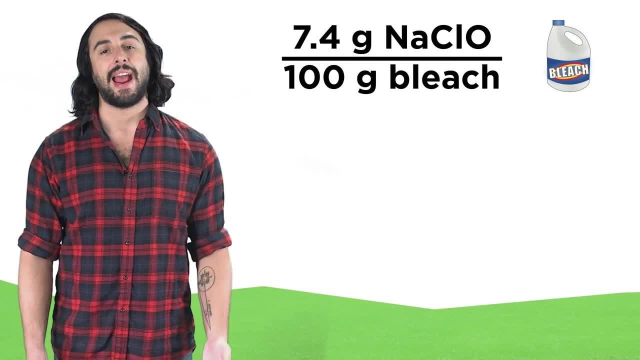 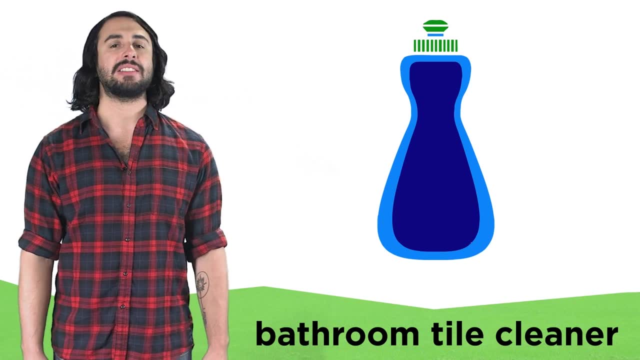 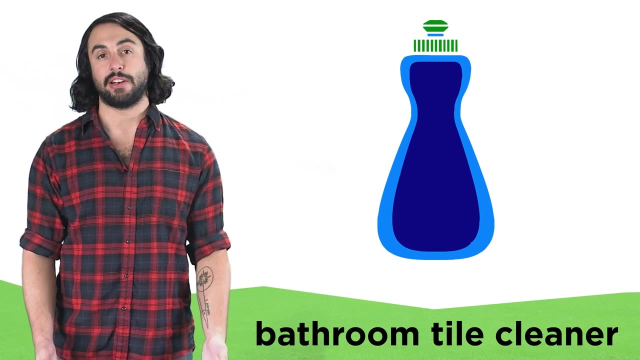 mass. 7.4 of those grams would be sodium hypochlorite and the rest would be water. In order to make sure we can calculate mass percentage, let's look at another household cleaning product. Let's say, a bottle of bathroom tile cleaner contains 165 grams of hydrochloric acid and 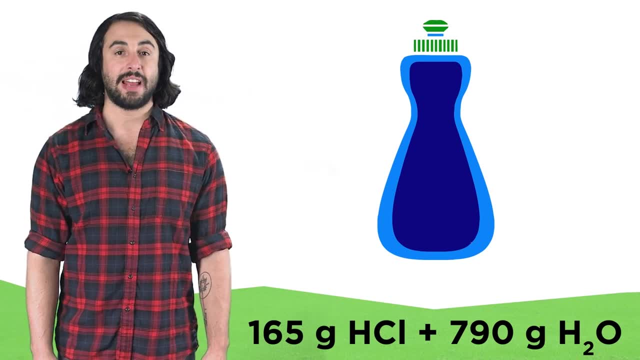 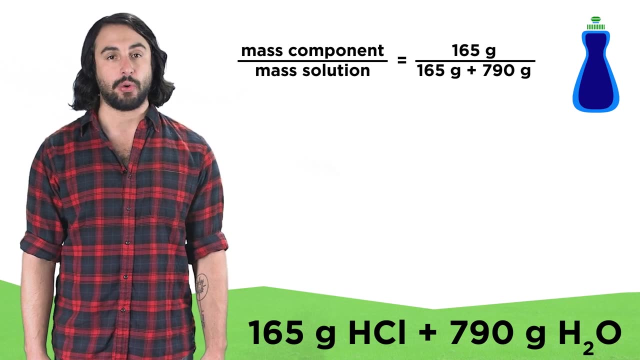 790 grams of water. What would be the percent mass of hydrochloric acid in this cleaner? Using our equation, we can plug in the mass of the component, in this case HCl, and the mass of the solution, which would be the sum of these masses. 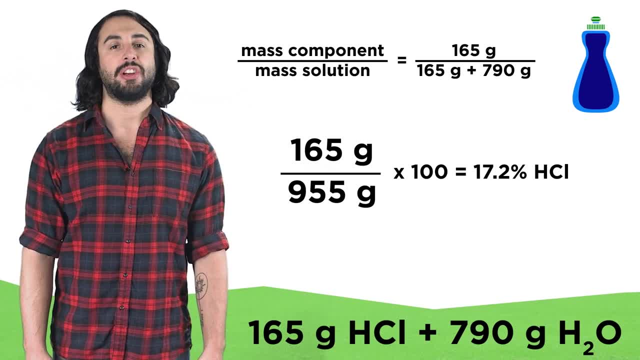 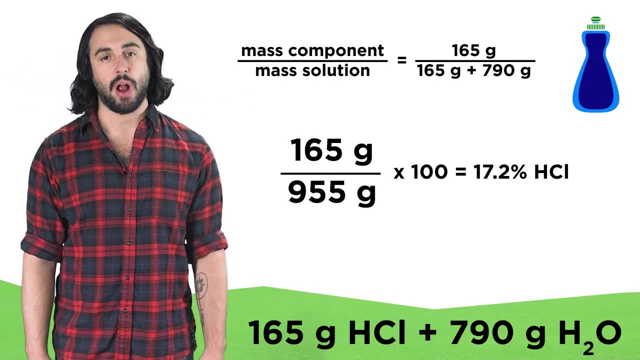 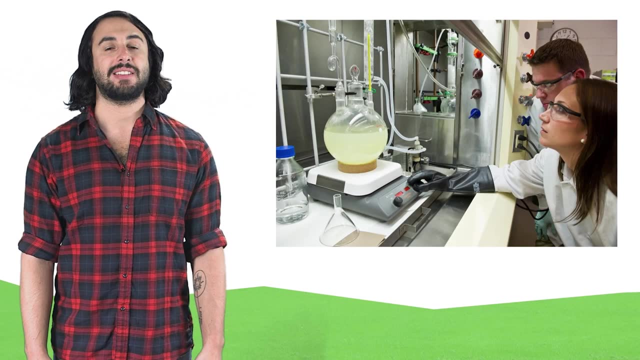 Then we divide and multiply the result by 100. We should get 17.2% as our answer. This is the mass percent of hydrochloric acid in the product, which we can then compare to other products if necessary. As we said, this concept is also useful in the long run. 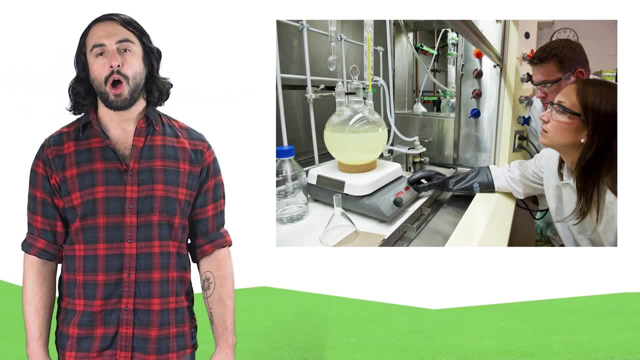 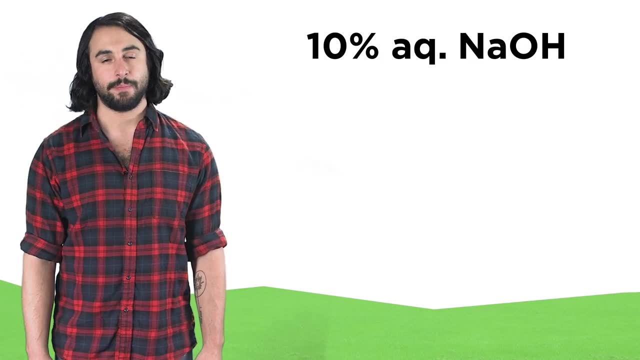 So let's look at another household cleaning product. Let's look at another household cleaning product. Let's look at another household cleaning product in the lab, because we won't always want to have to do stoichiometric calculations. If we want to make an aqueous solution that is 10% sodium hydroxide by mass, we could. 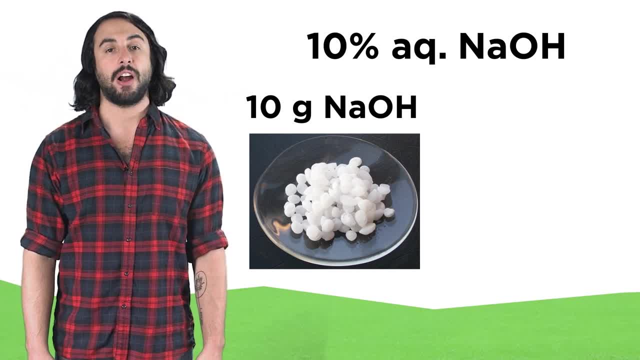 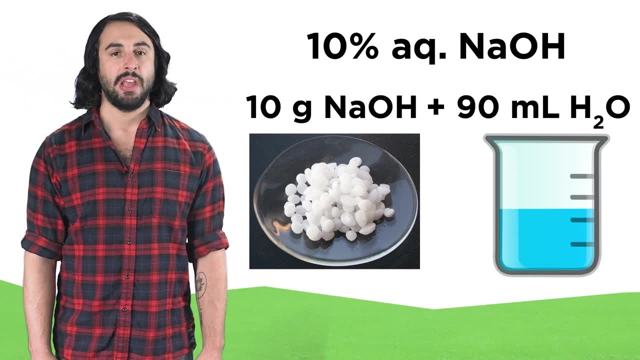 measure out 10 grams of sodium hydroxide pellets on a balance, place that in a flask and then simply add 90 milliliters of water, since water is precisely one gram per milliliter. 10 grams of sodium hydroxide. 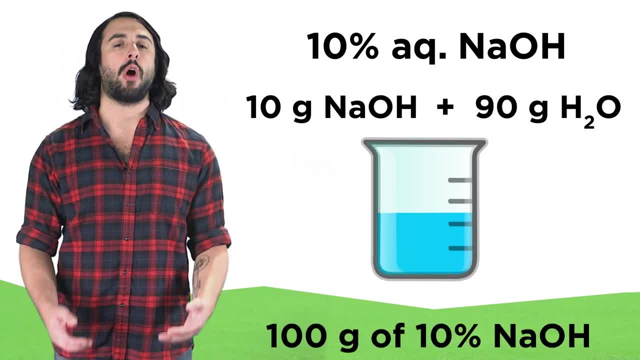 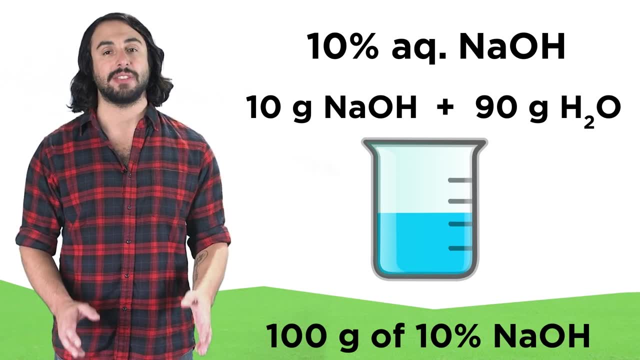 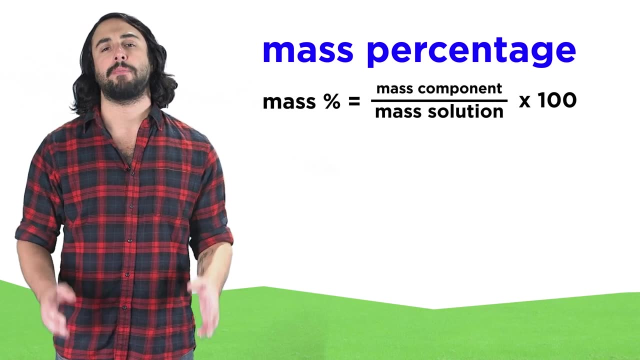 10 grams of sodium hydroxide plus 90 grams of water gives us a 100 gram solution, that is, 10% sodium hydroxide by mass, No calculations necessary. So we can see that this concept has a wide variety of applications, both for the public.